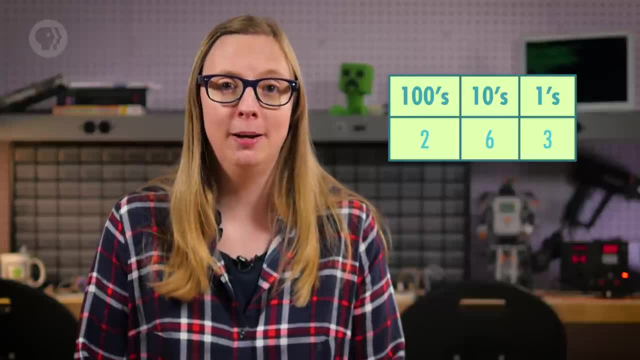 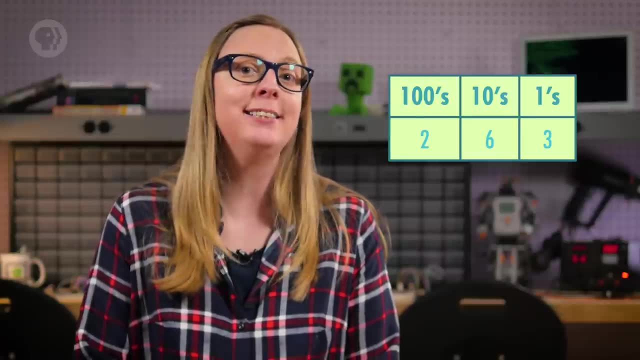 got 263.. Notice how each column has a different multiplier. In this case it's 100, 10 and 1.. Each multiplier is 10 times larger than the one to the right. That's because each column has 10 possible digits to work with: 0 through 9, after which. 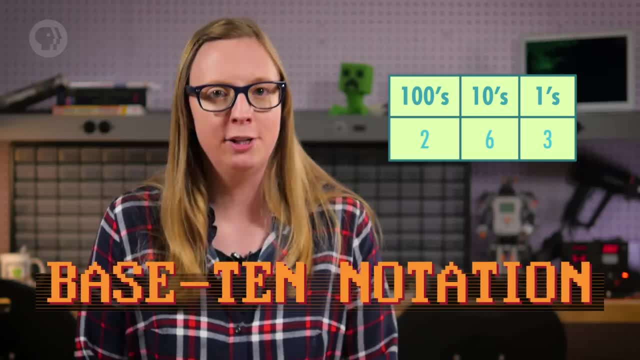 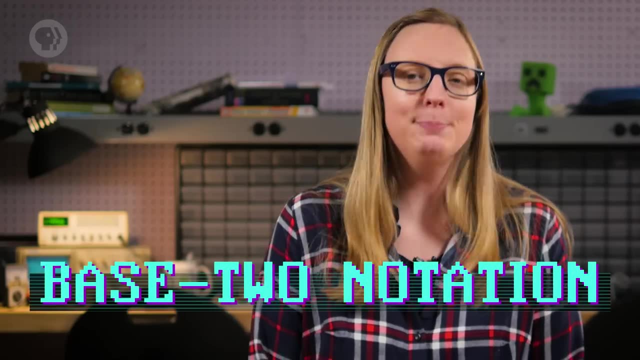 you have to carry one to the next column. For this reason it's called base 10 notation, also called decimal, since deci means 10.. And binary works exactly the same way, it's just base 2.. That's because there are only two possible digits in binary, 1 and 0.. 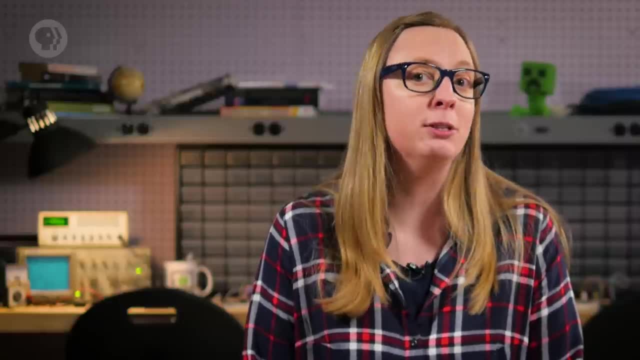 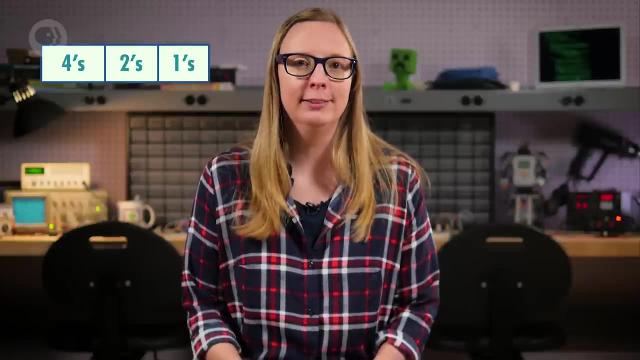 This means that each multiplier has to be 2 times larger than the column to its right. Instead of hundreds, tens and ones, we now have fours, twos and ones. Take, for example, the binary number 101.. This means we have one, four, zero twos and one one. 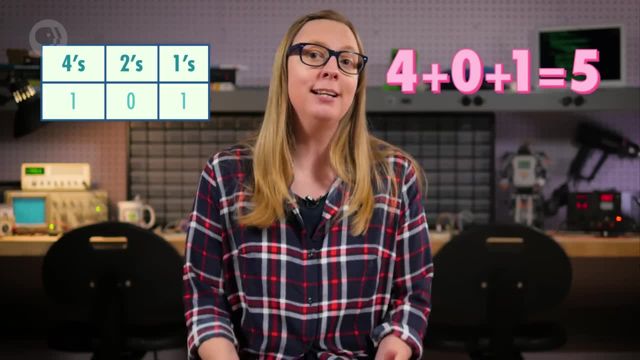 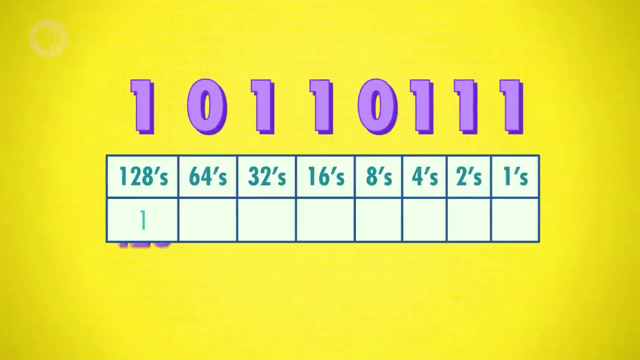 Add those all together and we've got the number 5 in base 10.. But to represent larger numbers, binary needs a lot more digits. Take this number in binary. We can convert it to decimal. in the same way. We have 1 times 128,, 0 times 64,, 1 times 32,, 1 times 16,, 0 times 8, 1 times 4, 1 times. 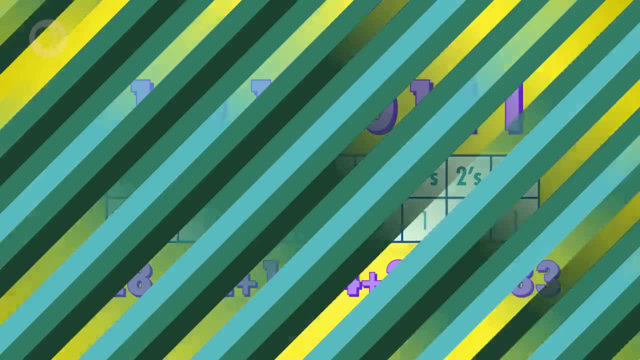 2, and 1 times 1,, which all adds up to 183.. Math with binary numbers isn't easy. It takes a lot of practice. It isn't hard either. Take, for example, decimal addition of 183 plus 19.. 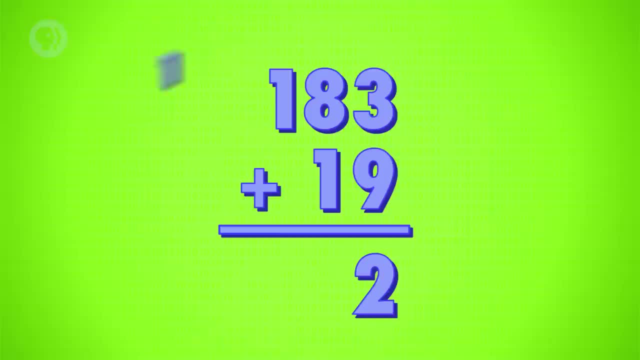 First we add 3 plus 9, that's 12.. So we put 2 as the sum and carry 1 to the tens column. Now we add 8 plus 1, plus the 1 we carried, that's 10.. 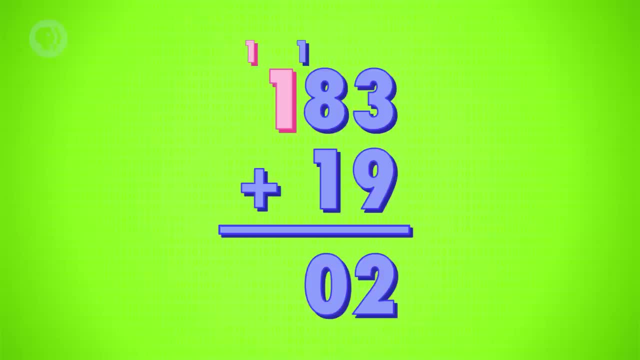 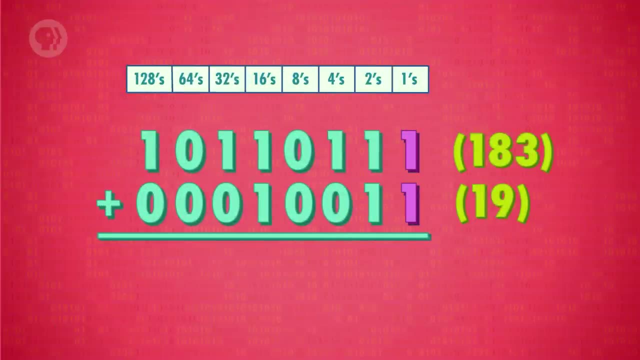 So the sum is 0, carry 1.. Finally, we add 1, plus the 1 we carried, which equals 2.. So the total sum is 202.. Here's the same sum, but in binary, Just as before we start with the ones column. 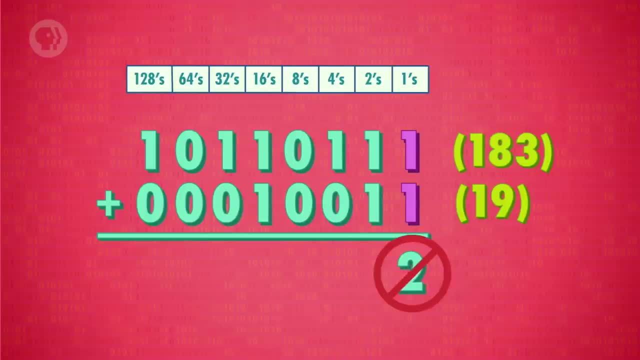 Adding 1 plus 1 results in 2,, even in binary, But there is no symbol 2.. We add 1, 0 and put 0 as our sum and carry the 1.. Just like in our decimal example: 1 plus 1 plus the 1 carried equals 3, or 1, 1 in binary. 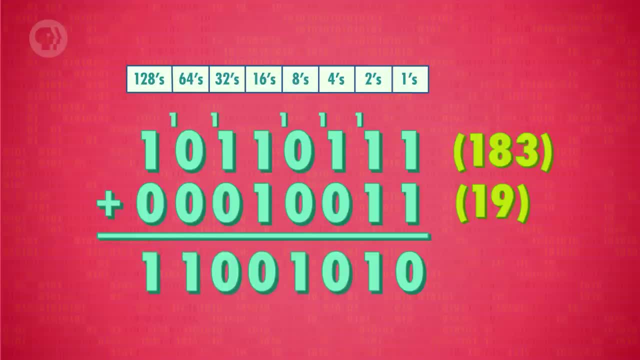 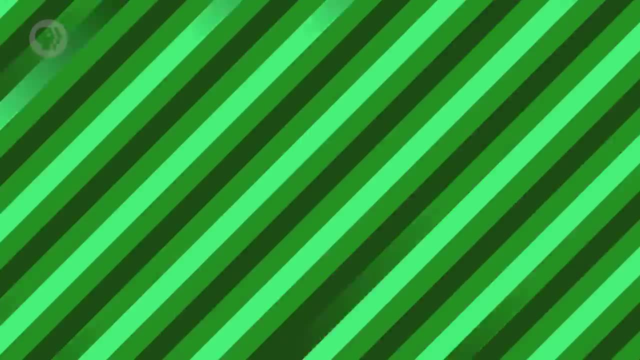 So we put the sum as 1 and carry 1 again and so on. We end up with this number, which is the same as the number 202 in base 10.. Each of these binary digits- 1 or 0, is called a bit. 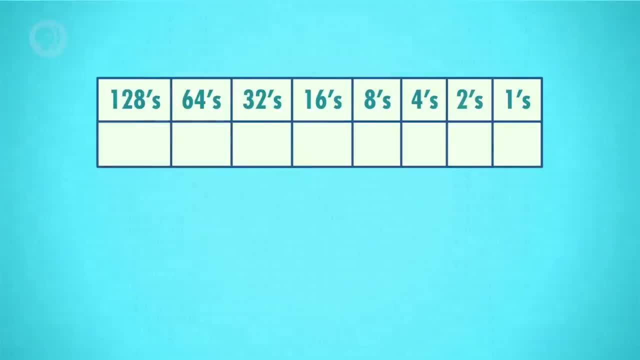 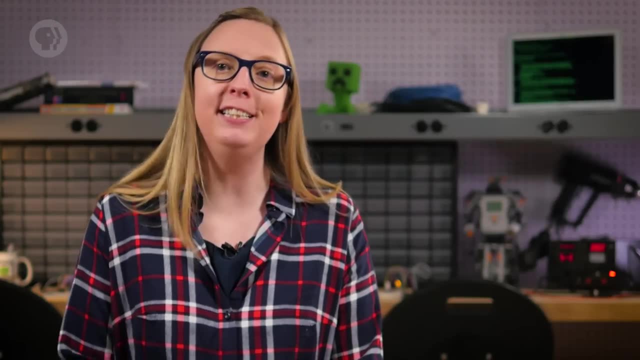 So in these last few examples, we were using 8-bit numbers, with their lowest value of 0 and highest value of 255, which requires all 8 bits to be set to 1.. That's 256 different values, or 2 to the 8th power. 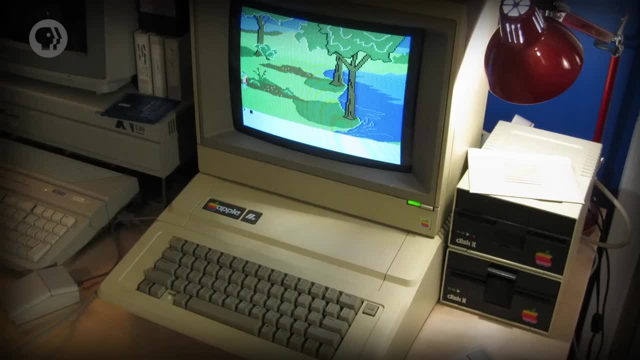 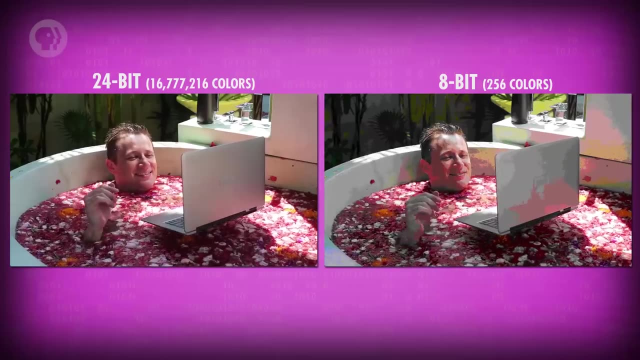 You might have heard of 8-bit computers or 8-bit graphics or audio. These were computers that did most of their operations in chunks of 8 bits, But 256 different values isn't a lot to work with, So it meant things like 8-bit games were limited to just 256 different colors for their graphics. 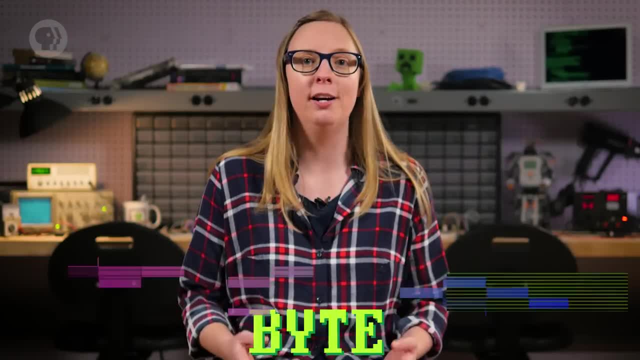 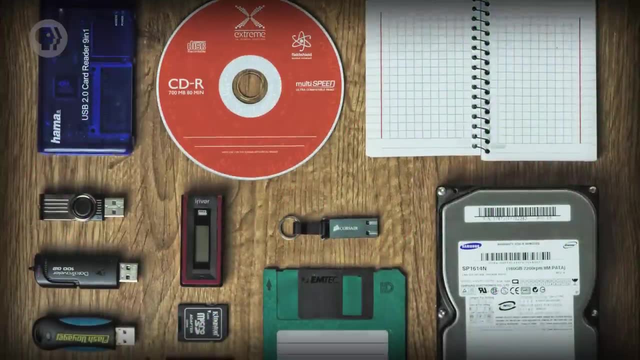 And 8 bits is such a common size in computing it has a special word: a byte. A byte is 8 bits. If you've got 10 bytes, it means you've really got 80 bits. You've heard of kilobytes, megabytes. 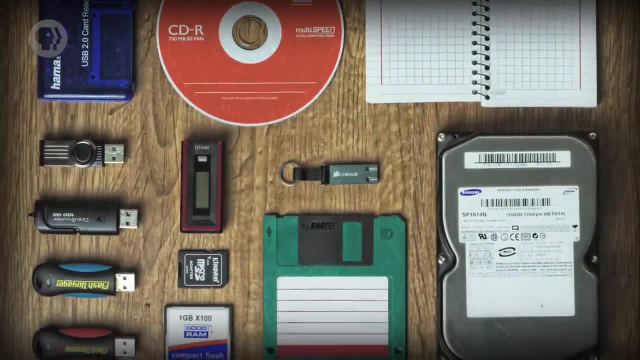 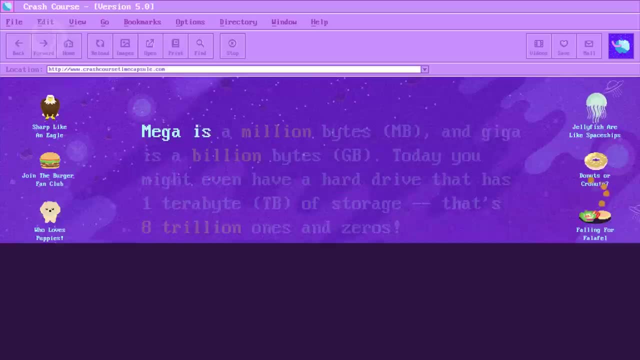 Gigabytes and so on. These prefixes donate different scales of data. Just like 1 kilogram is 1000 grams, 1 kilobyte is 1000 bytes, or really 8000 bits, Mega is a million bytes and giga is a billion bytes. 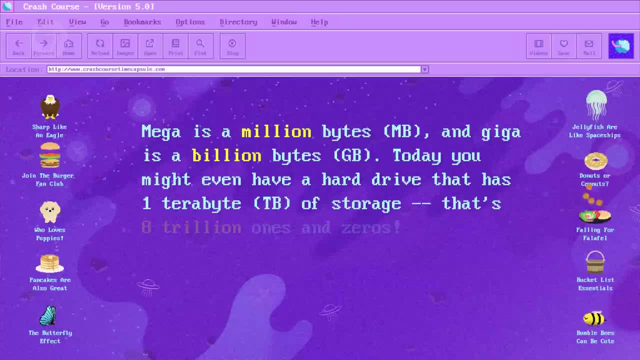 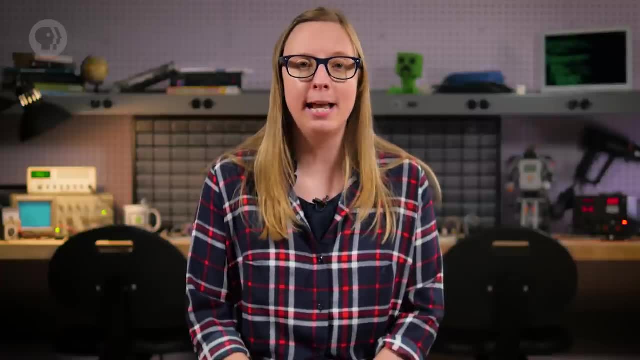 Today you might even have a hard drive that has 1 terabyte of storage. That's 8 trillion ones and zeros. But hold on, that's not always true. In binary, a kilobyte has 2 to the power of 10 bytes, or 1024. 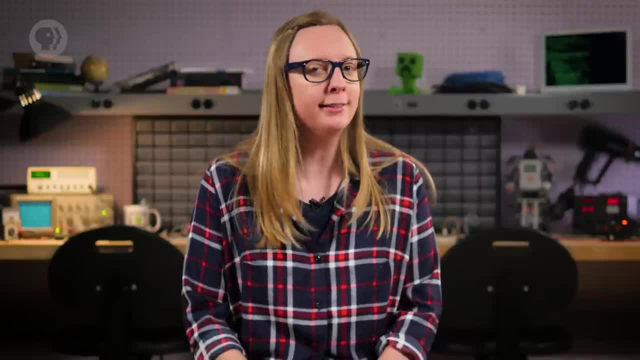 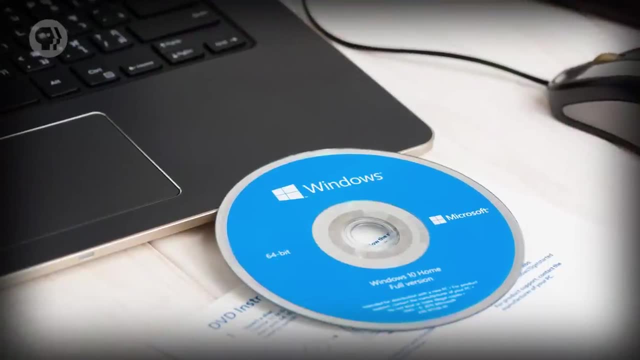 A thousand is also right when talking about kilobytes, But we should acknowledge it isn't the only correct definition. You've probably also heard the term 32-bit or 64-bit computers. You're almost certainly using one right now. What this means is that they operate in chunks of 32 or 64 bits. 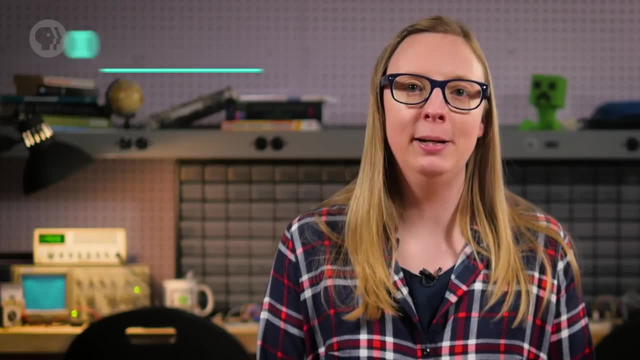 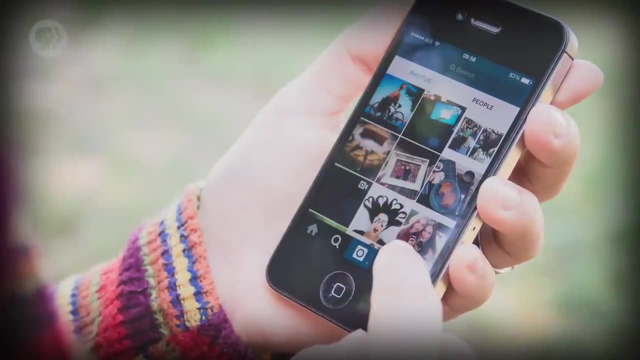 That's a lot of bits. The largest number you can represent with 32 bits is just under 4.3 billion, which is 32 ones in binary. This is why our Instagram photos are so smooth and pretty. They are composed of millions of colors, because computers today use 32-bit color graphics. 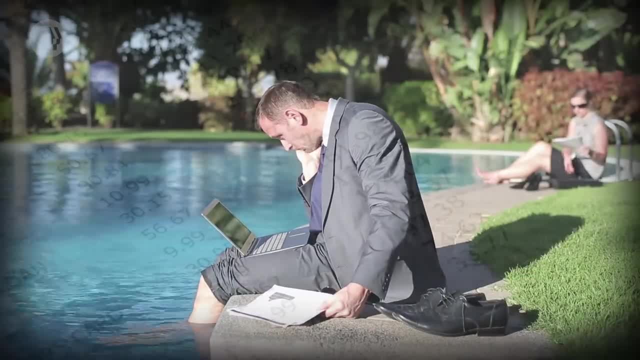 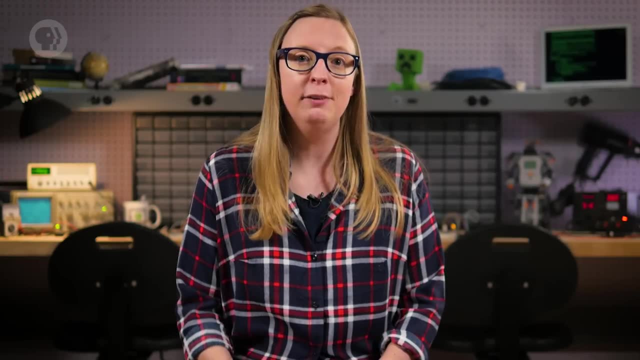 Of course, not everything is a positive number, like my bank account in college, So we need a way to represent positive and negative numbers. Most computers use the first bit for the sign, 1 for negative, 0 for positive numbers and. 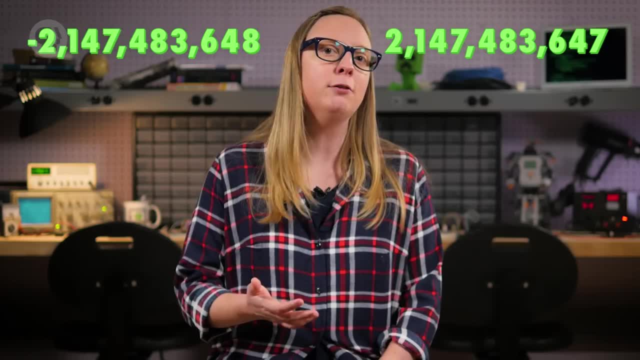 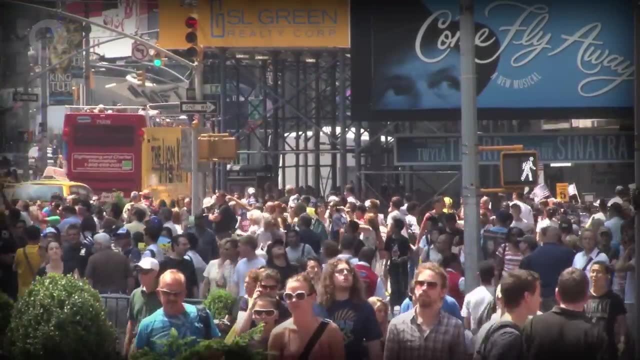 then use the remaining 31 bits for the number itself. That gives us a range of roughly plus or minus 2 billion. While this is a pretty big range of numbers, it's not enough for many tasks. There are 7 billion people on the Earth and the US national debt is almost 20 trillion. 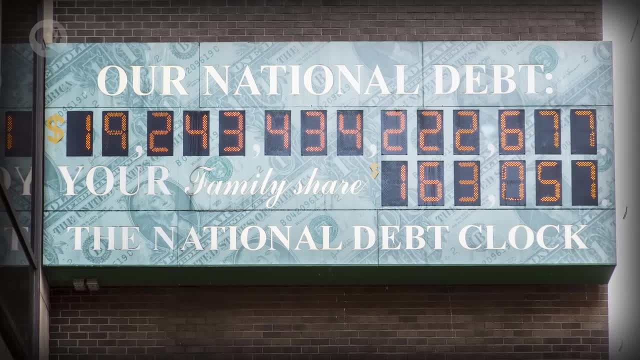 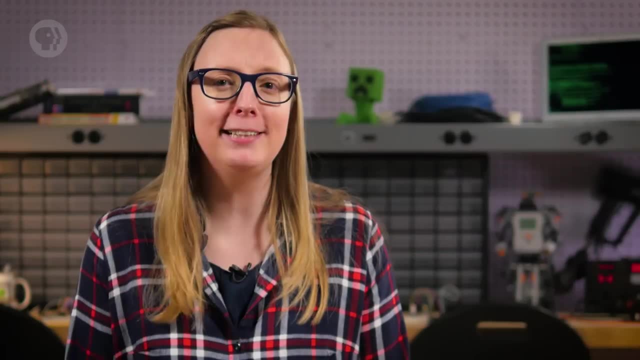 dollars after all. This is why 64-bit numbers are useful. The largest value a 64-bit number can represent is around 9.2 quintillion. That's a lot of possible numbers and will hopefully stay above the US national debt for a while. 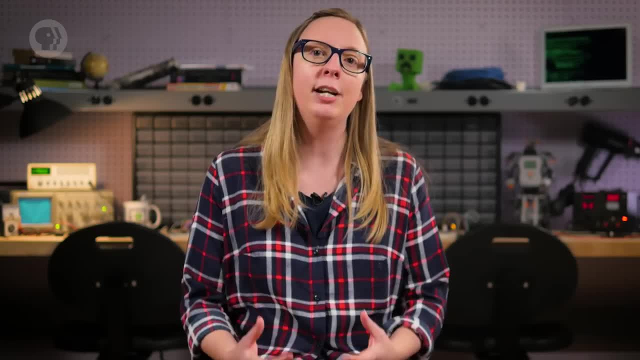 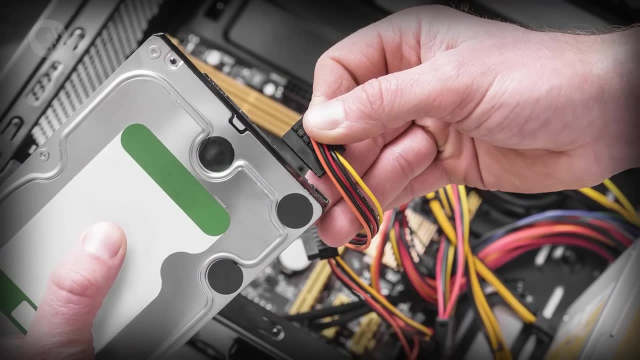 Most importantly, as we'll discuss in a later episode, computers must label locations in their memory, known as addresses, in order to store and retrieve values, As computer memory has grown to gigabytes and terabytes, that's trillions of bytes. 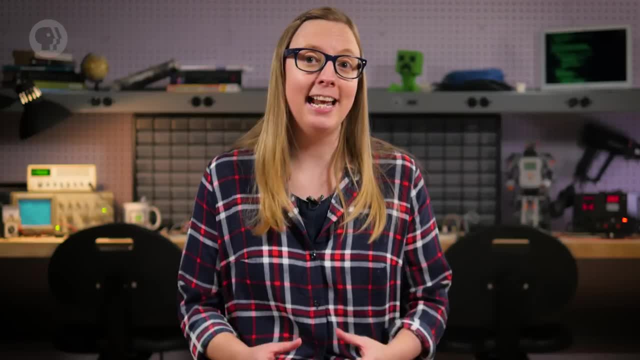 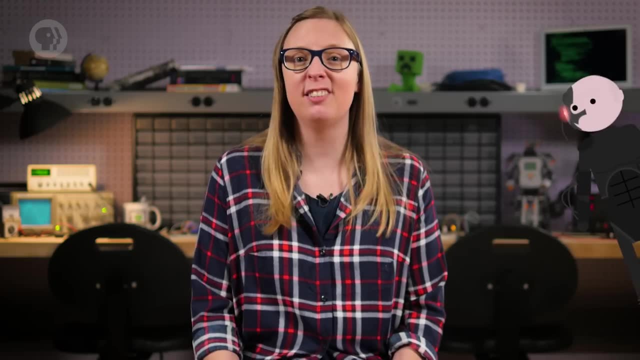 it was necessary to have 64-bit memory addresses as well. In addition to negative and positive numbers, computers must deal with numbers that are not whole numbers: 1.7 and 3.14, or maybe even stardate 43989.1.. 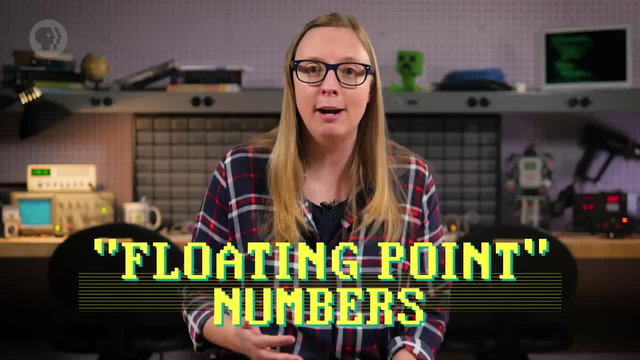 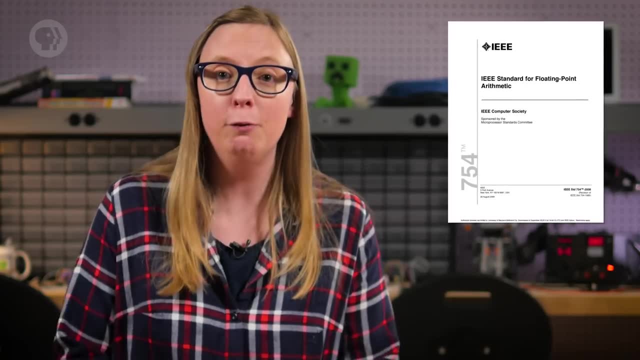 These are called floating-point numbers because the decimal point can float around in the middle of a number. Several methods have been developed to represent floating-point numbers, the most common of which is the IEEE 754 standard. and you thought historians were the only people bad at naming. 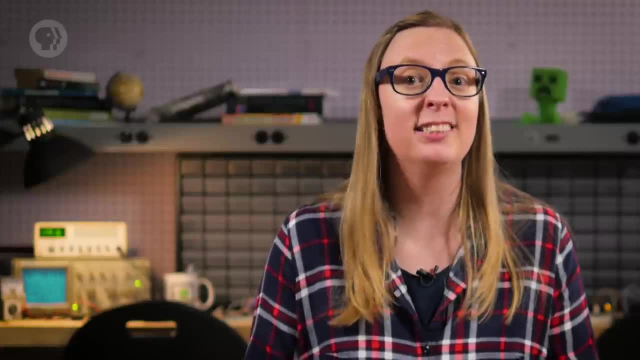 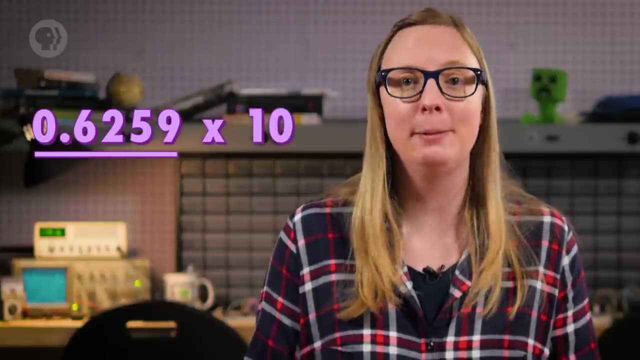 things. In essence, this standard stores decimal values, sort of like scientific notation. For example, 625.9 can be written as 0.6259 times 10 to the power of 3.. That's a lot of possible numbers. There are two important numbers here. 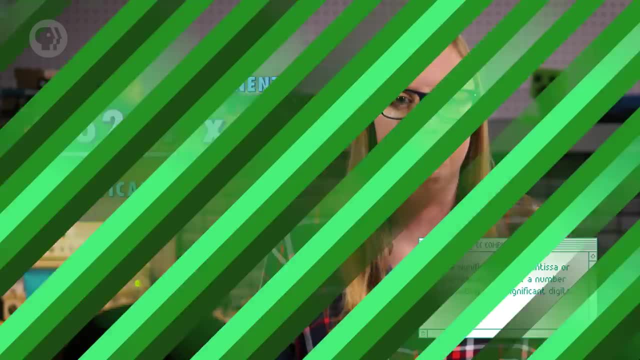 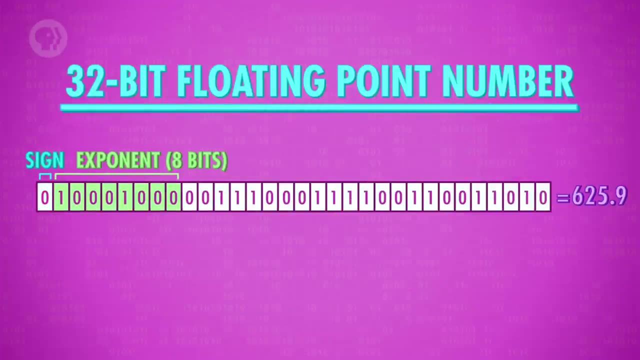 The point 6259 is called the significant and 3 is the exponent In a 32-bit floating-point number. the first bit is used for the sign of the number positive or negative, The next 8 bits are used to store the exponent and the remaining 23 bits are used to store. 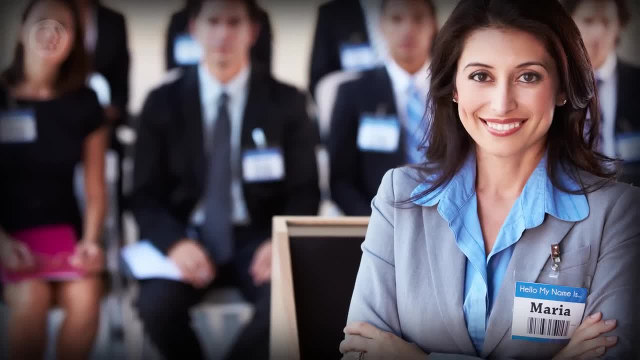 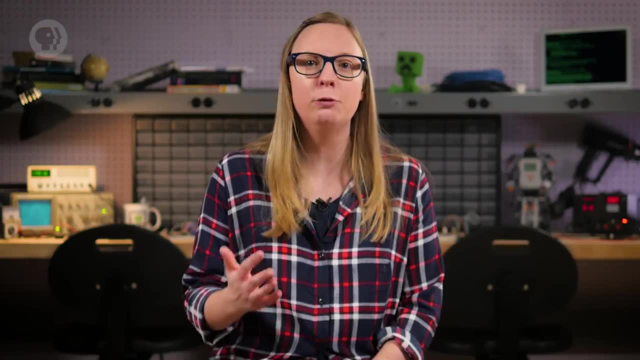 the significant. OK, we've talked a lot about numbers, but your name is probably composed of letters, so it's really useful for computers to also have a way to represent text. However, rather than have a special form of storage for letters, computers simply use: 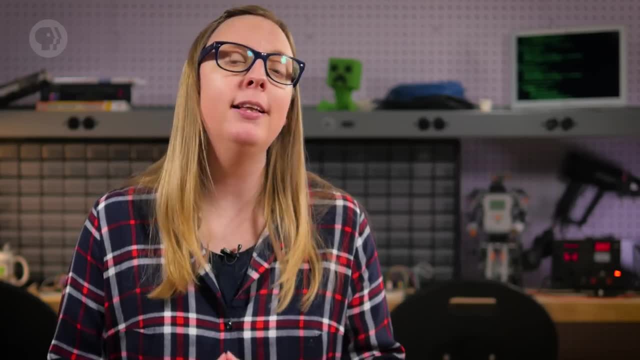 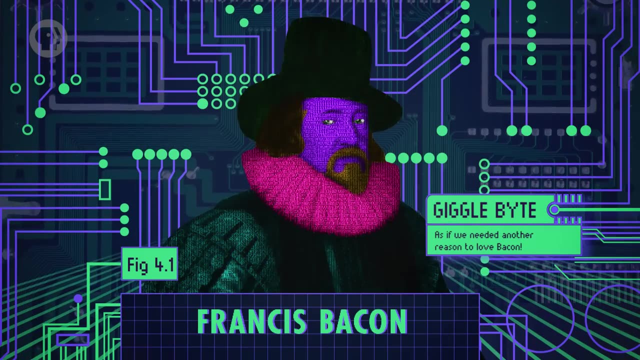 to represent letters. The most straightforward approach might be to simply number the letters of the alphabet: A being 1,, B being 2,, C, 3, and so on. In fact, Francis Bacon, the famous English writer, used 5-bit sequences to encode all. 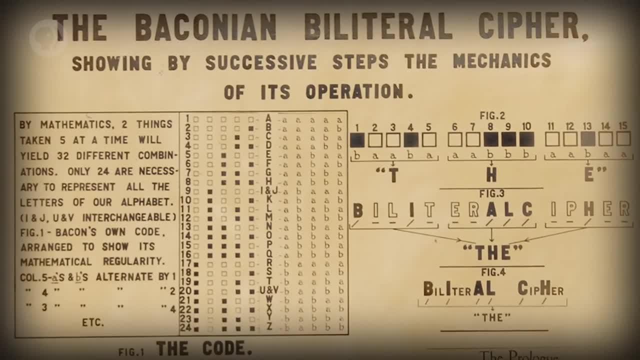 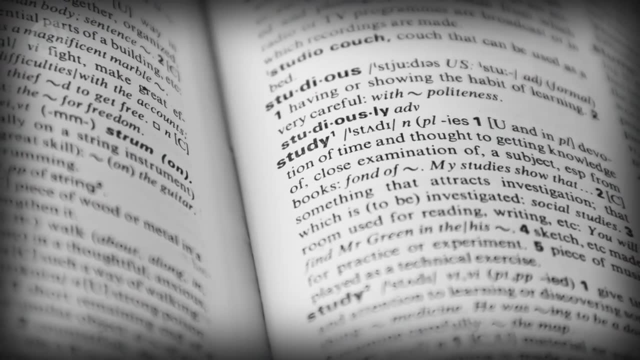 26 letters of the English alphabet to send secret messages back in the 1600s, And 5 bits can store 32 possible values. so that's enough for the 26 letters, but not enough for punctuation digits and upper and lowercase letters. 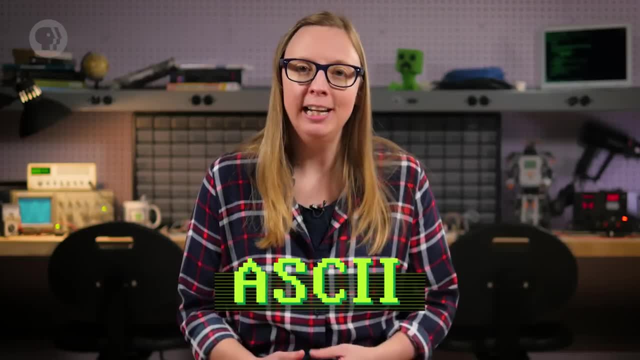 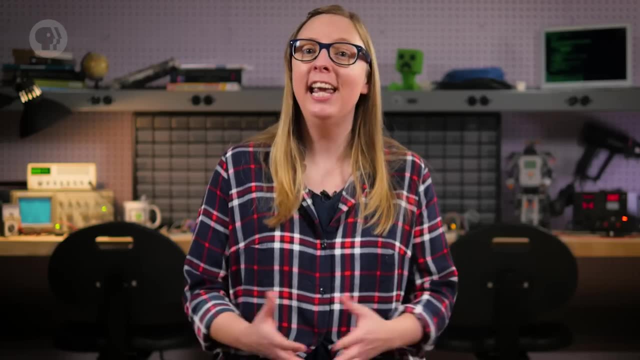 Enter ASCII, the American Standard Code for Information Interchange. Invented in 1963,, ASCII was a 7-bit code, enough to store 128 different values. With this expanded range, it could encode capital letters, lowercase letters, digits 0 through 9, and symbols like the at sign and punctuation marks. 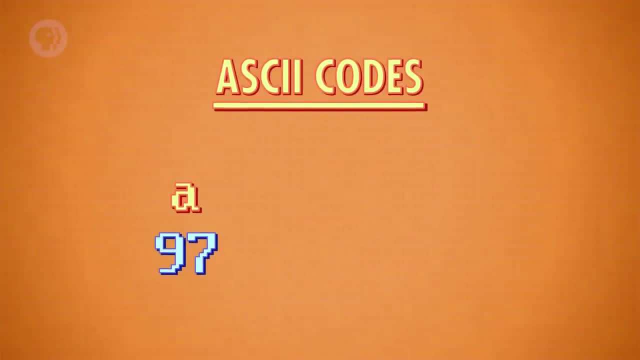 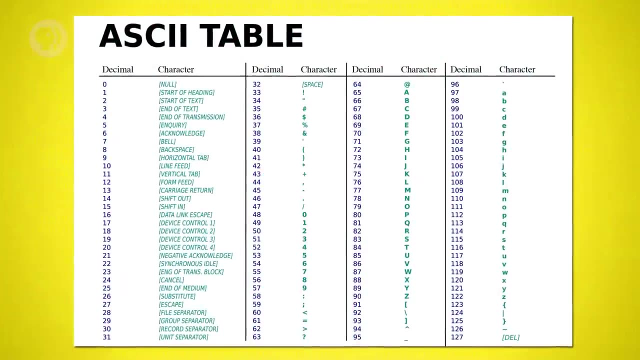 For example, a lowercase a is represented by the number 97,, while a capital A is 65,, a colon is 58, and a closed parenthesis is 41.. ASCII even had a selection of special command codes, such as a newline character, to tell. 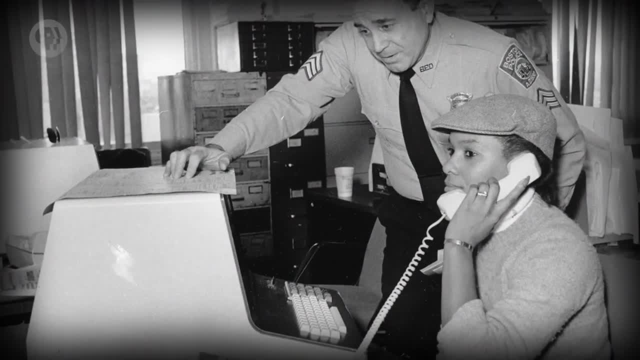 the computer where to wrap a line to the next row. In older computer systems the command line was called ASCII. It was the same as ASCII. The line of text would literally continue off the edge of the screen if you didn't include a newline character. 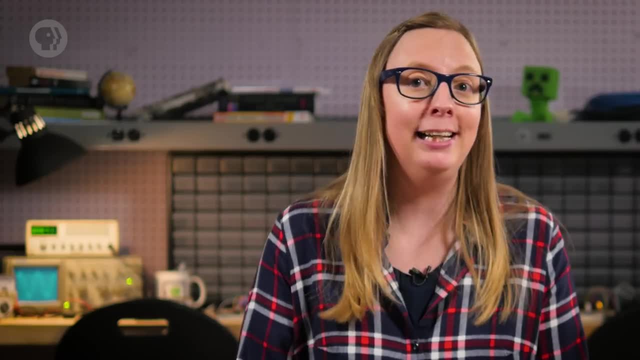 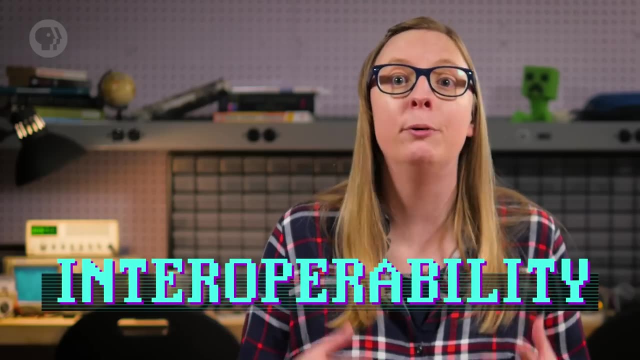 Because ASCII was such an early standard, it became widely used and critically allowed different computers built by different companies to exchange data. This ability to universally exchange information is called interoperability. However, it did have a major limitation: It was really only designed for English. Fortunately, there are 8 bits in a byte, not 7, and it soon became popular to use codes 128 through 255, previously unused for national code. In the US, those extra numbers were largely used to encode additional symbols like mathematical. 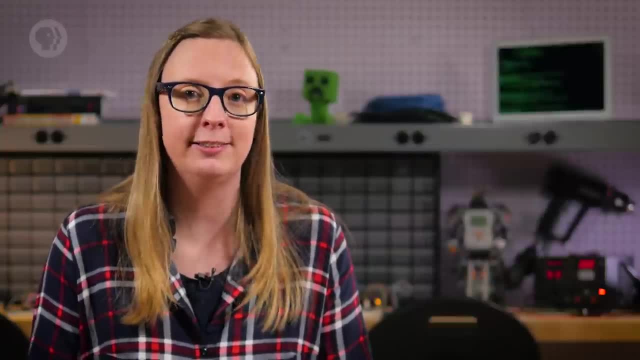 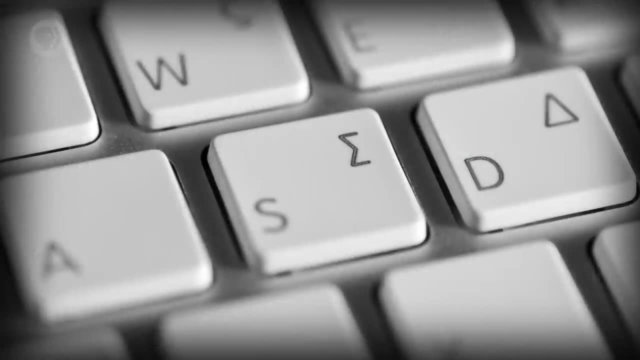 notation, graphical elements and common accentuated characters. On the other hand, while the Latin characters were used universally, Russian computers used the extra codes to encode Cyrillic characters and Greek computers Greek letters and so on, And national character codes worked pretty well for most countries. 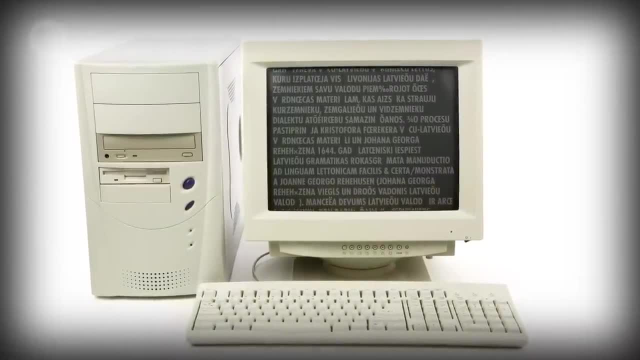 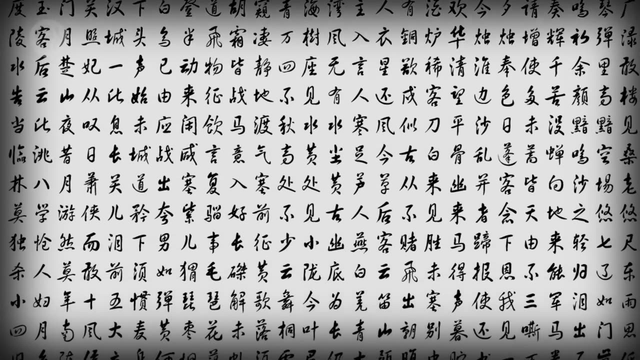 The problem was if you opened an email written in Latvian on a Turkish computer, the result was completely incomprehensible And things totally broke with the rise of ASCII. As languages like Chinese and Japanese have thousands of characters, there was no way. 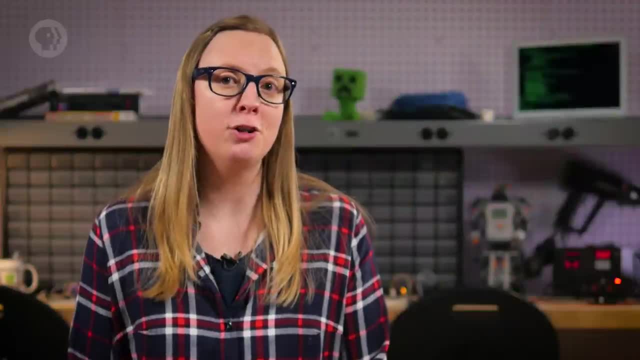 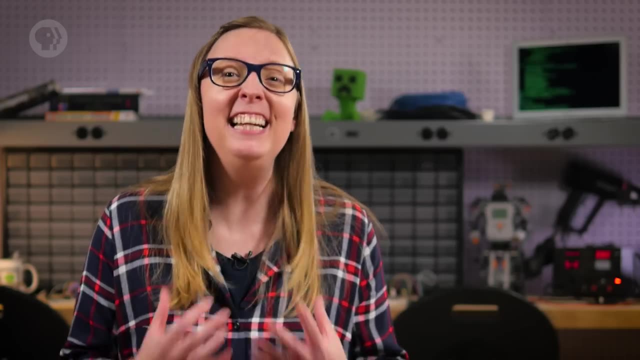 to encode all those characters in 8 bits. In response, each country invented multi-byte encoding schemes, all of which were mutually incompatible. The Japanese were so familiar with this encoding problem that they even had a special name for it – Mojibake, which means scrambled text. 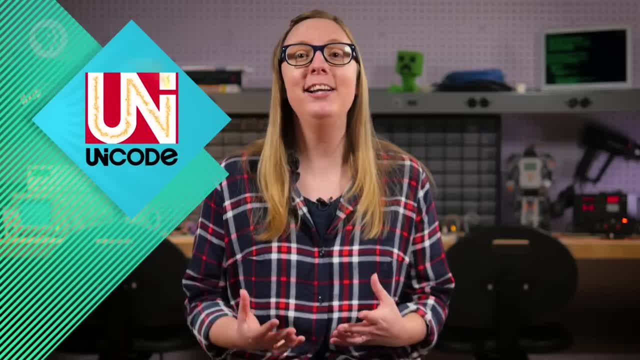 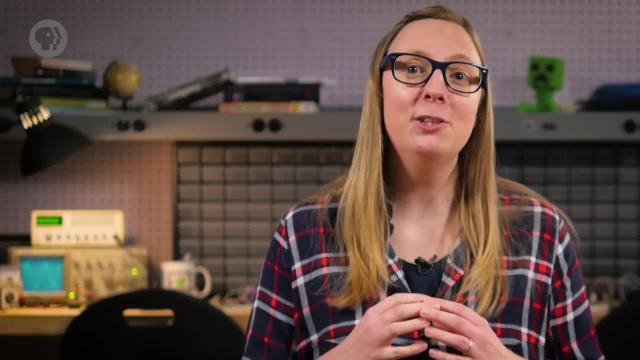 And so it was born: Unicode, one format to rule them all. Devised in 1992 to finally do away with all of the different international schemes, it replaced them with one universal code. The most common version of Unicode uses 16 bits with space for over a million codes. 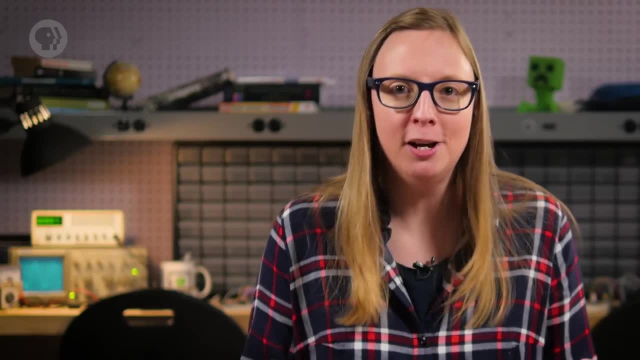 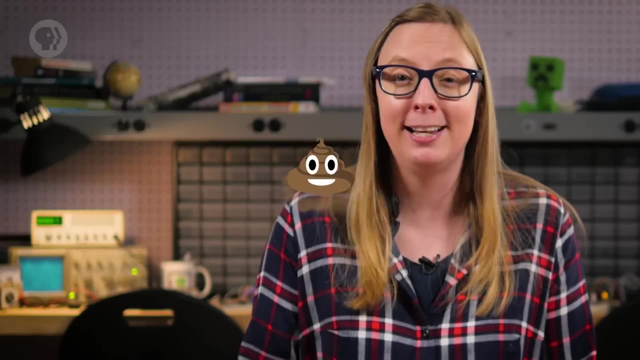 – enough for every single character from every language ever used, More than 120,000 of them in over a hundred types of script, plus space for mathematical symbols and even graphical characters like emoji. And in the same way that ASCII defines a scheme for encoding letters as binary numbers, other 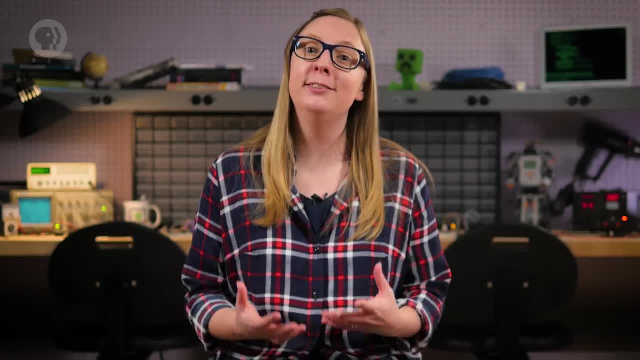 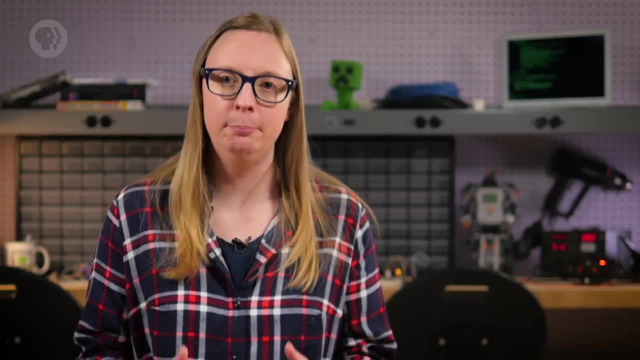 file formats like MP3s or GIFs use binary numbers to encode sounds or colors of a pixel in our photos, movies and music. Most importantly, under the hood, it all comes together, And that's why ASCII is so important, Because it all comes down to long sequences of bits.